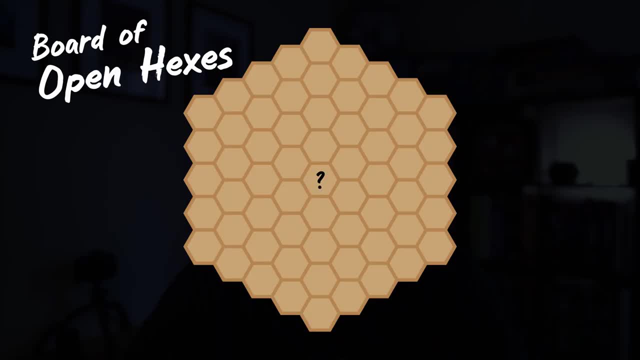 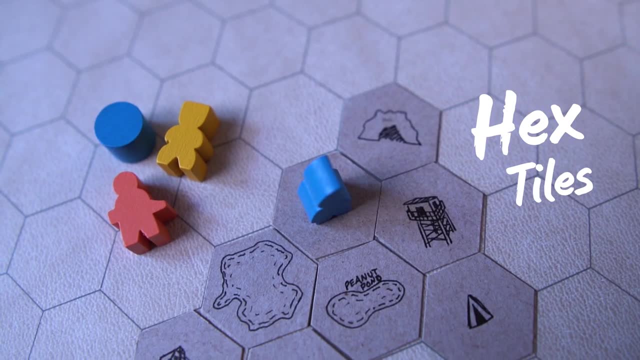 So here's what my game includes, just so you're caught up. Right now my game includes a blank board of open hex spaces, you know, big enough to put my hopes and dreams. That brings me to the unique hex tiles with explorable locations and actions. Hopefully players will learn. 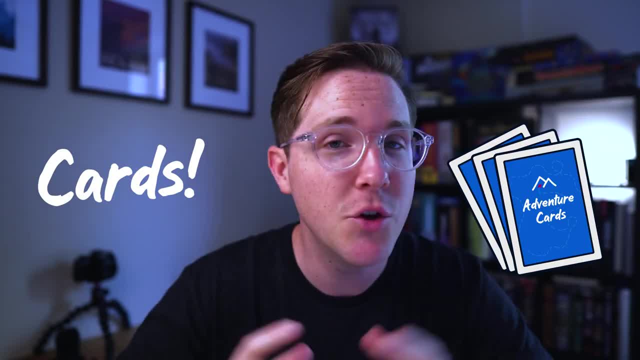 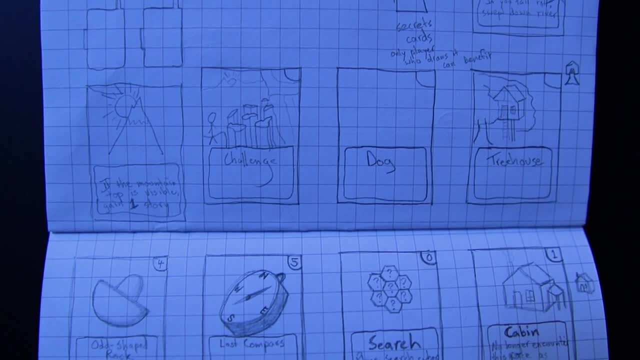 to love these. I already do Cards, the kind that you can find in an adventure deck. These will probably be the main driver of narrative for my game, but I am also very confident that there are other elements of the game that will stand on their own in how they help create narrative, If you have any. 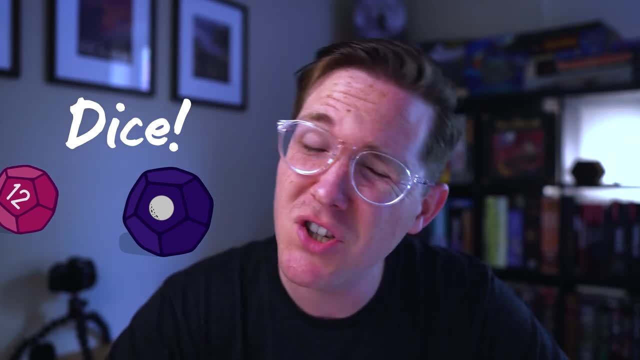 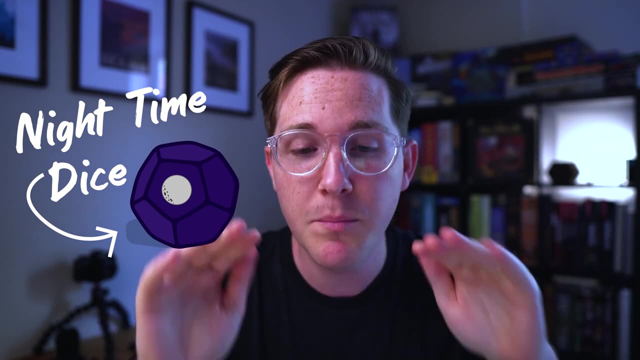 ideas, please let me know in the comments. Dice: Possibly two, maybe just one, At least one dice for the night time events. This dice only has good things on it. nothing bad Only benefits During the night time phase one. 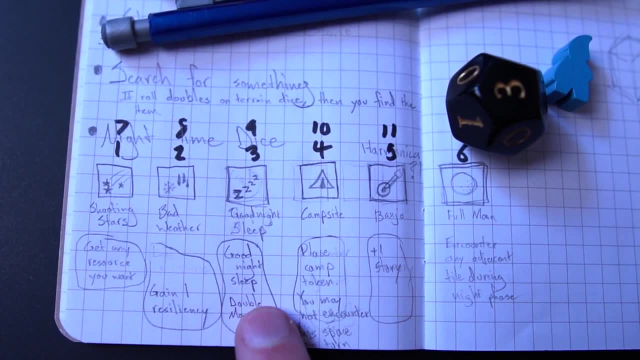 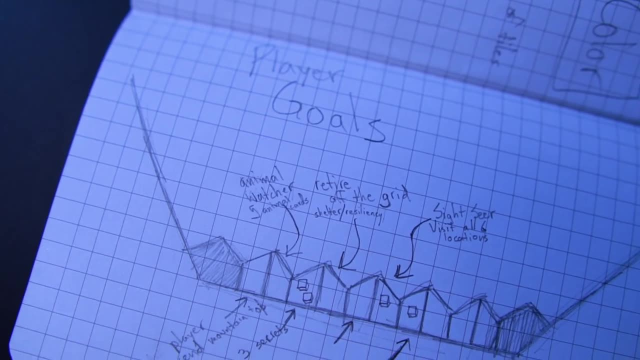 player rolls this dice and all players find out what the benefit or opportunity is for that phase. Individual player goals: These are the winning conditions of the game. If a player achieves all of their personal goals in the game, they win And they go home satisfied and feeling. 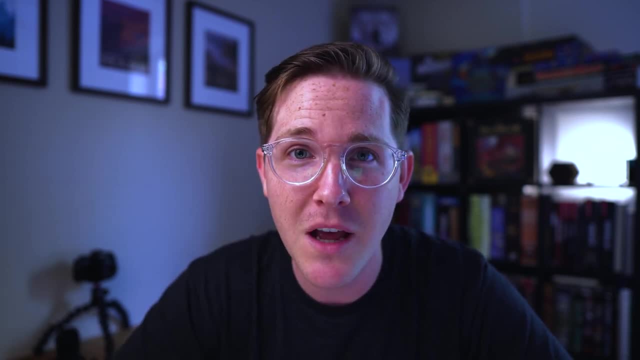 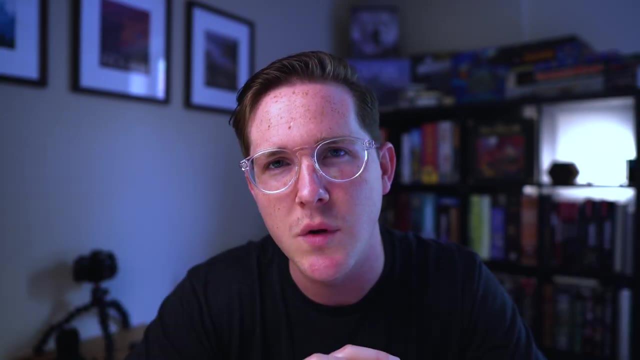 accomplished. It took them a long time to get to the top of the mountain, but at least they set a goal and they did it, And by golly they did it. This is the ensemble of mechanisms, components and rules I have so far. They're incomplete. 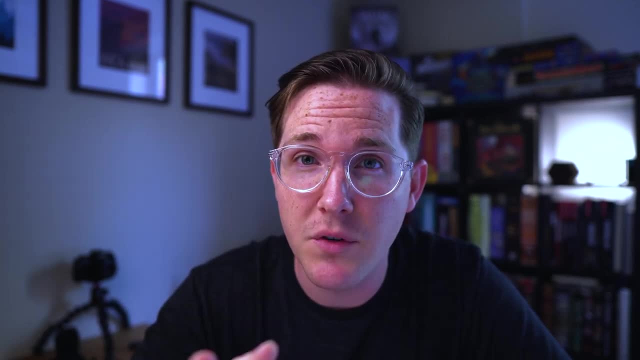 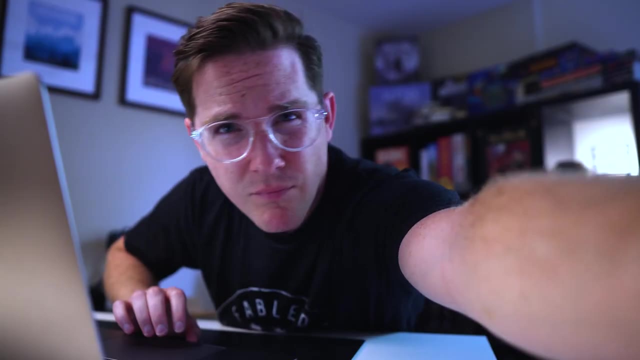 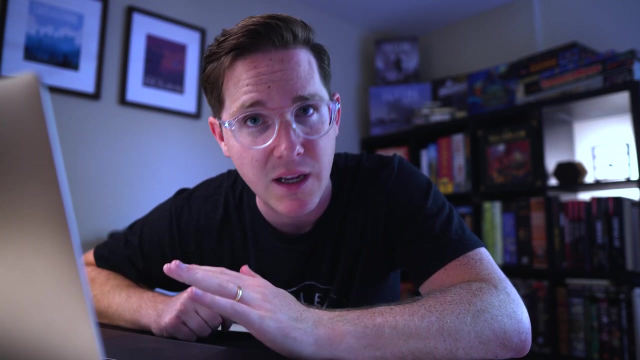 for sure, but they're a good start and definitely a solid foundation for the development process to come. There are other games that deserve mentioning before I get into the narrative of my game, especially since these published games have similarities in the theme and mechanisms. 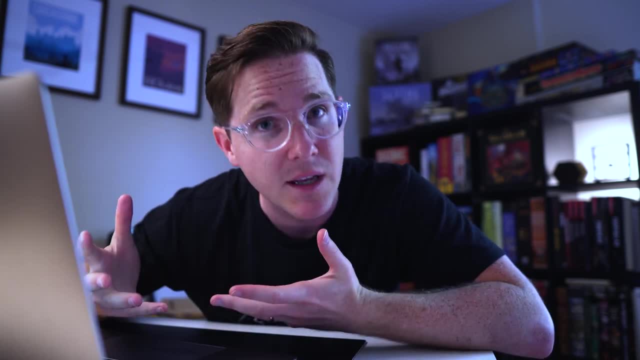 and since it's felt like I've been talking about these games for a long time, I'm going to start talking around them for the last few videos, without meaning to. These games also offer narrative, so it would be good to distinguish how my game creates. 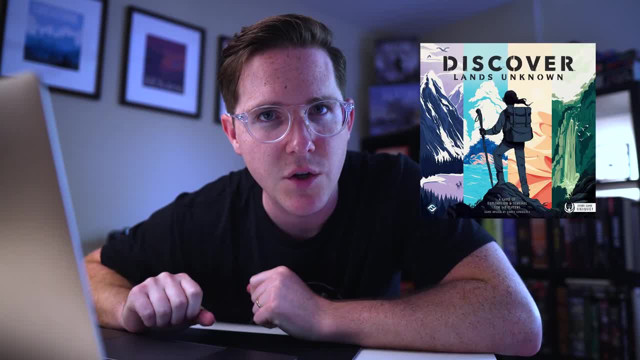 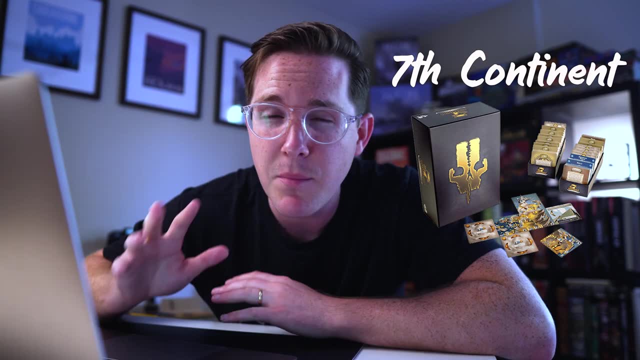 narrative in a different way. I've already discussed Discover Lands Unknown in a different video, so I won't cover it here. There's even another game in the same exploration genre called Seventh Continent. This game also uses a numbered adventure deck that helps deliver events, items and story beats. 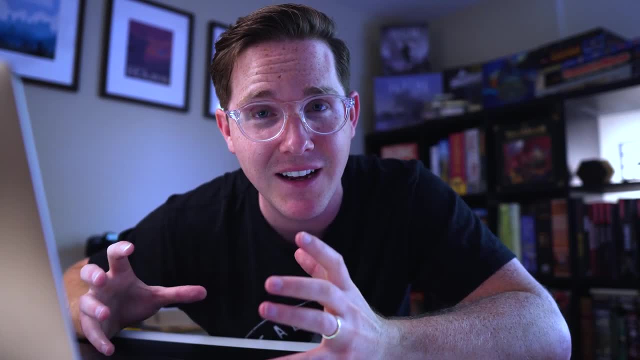 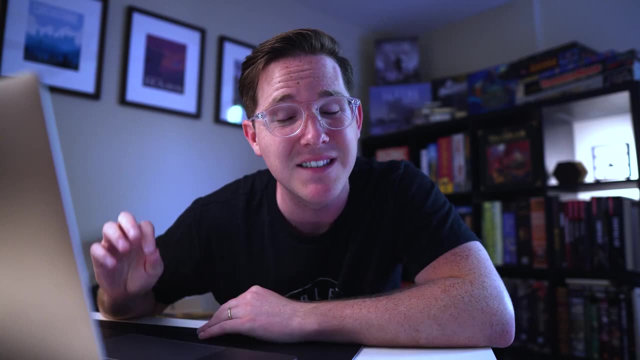 I'm not smart enough to mastermind a 400 card event deck in order to create narrative, so there shouldn't be any threat. That's why I did it for the video. So let's get started of overlap here. The next game has been brought up the most due to its apparent 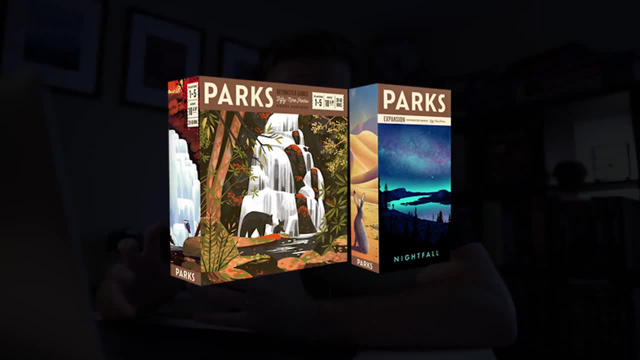 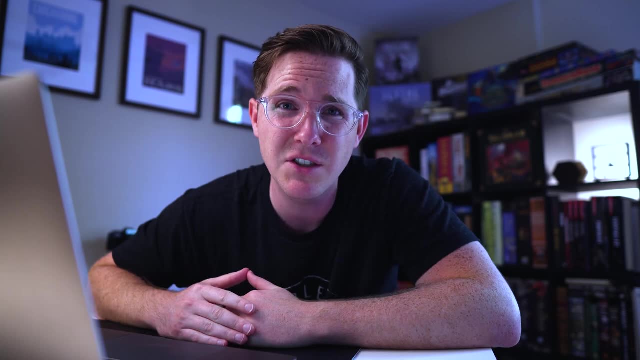 similar theme to mine. That game is Parks. Parks is a great game and I know Keymaster Games just released a new expansion for Parks because people loved it so much. I honestly should have Parks in my collection because the theme is right up my alley. I actually used to work for a college program that took students on. 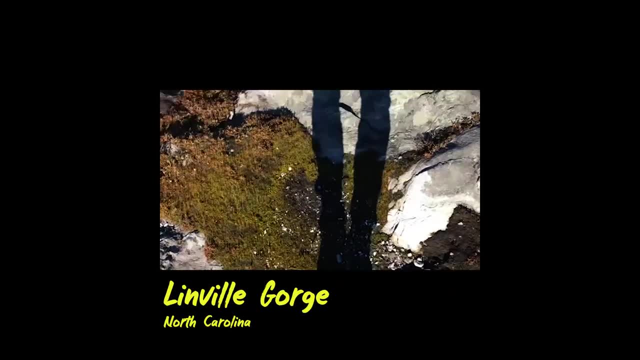 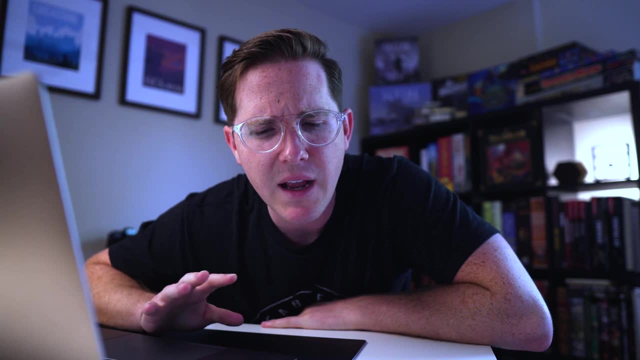 outdoor trips for hiking, camping and climbing. I'm an outdoorsy person at heart and I love traveling to national parks and experiencing what the outside world has to offer. But maybe that's why I haven't gravitated towards the gameplay of Parks yet, Because even though the amazing art does everything, 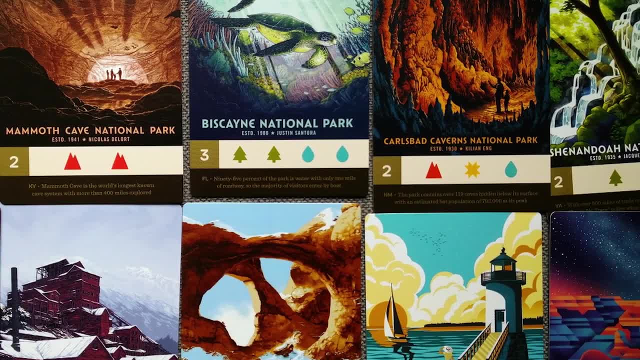 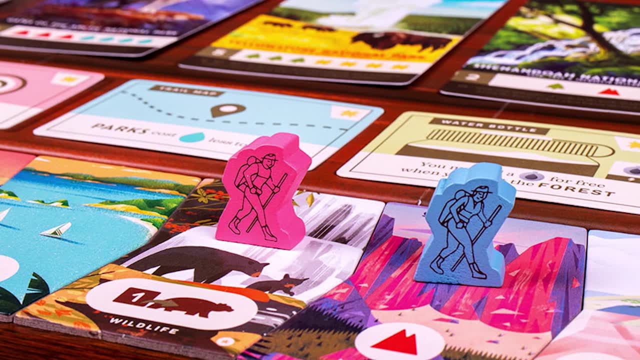 it can to illustrate an atmosphere of hiking through beautiful national parks and getting players to cherish the great outdoors. the gameplay is more abstract than what I would want to play on a regular basis. Parks is more about set collection and moving your hikers along a linear track to take actions before. 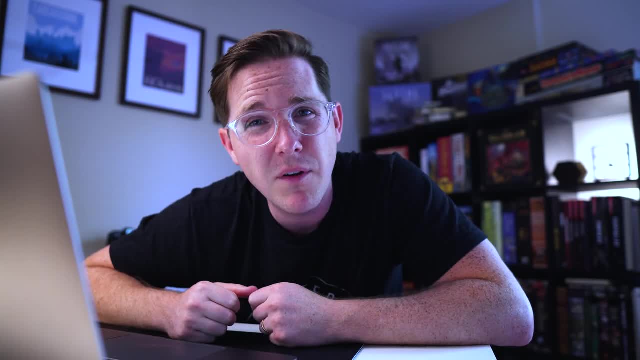 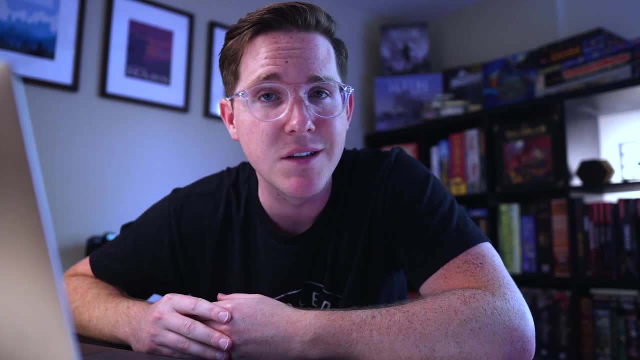 they run out. The game works really well, but maybe it doesn't go far enough in the adventure aspect for me. The last game I'll mention is Robinson Crusoe, another well-known game. Gotta admit, I've never played this one and once I got that first message that it was apparently similar and how it. 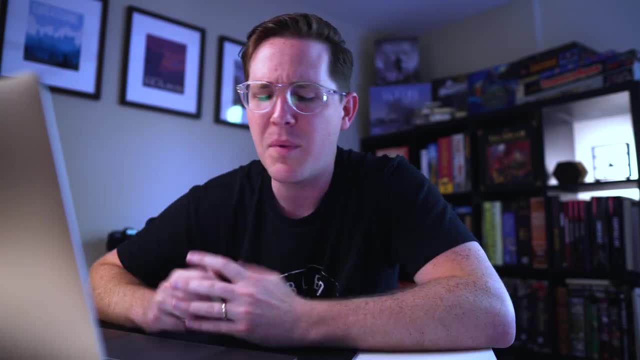 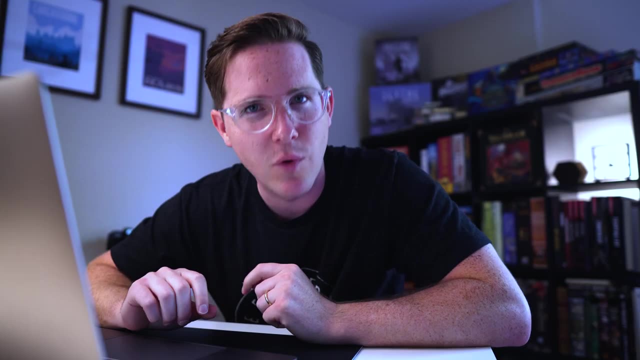 uses hex tiles for exploration. I got a little nervous, But then I remembered I'm not designing a Robinson Crusoe game, I'm designing my game. and that was enough to put me at rest Because, remember, I'm aiming for a specific feeling in my game. 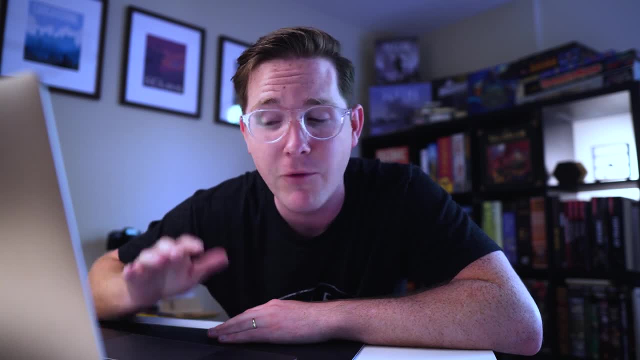 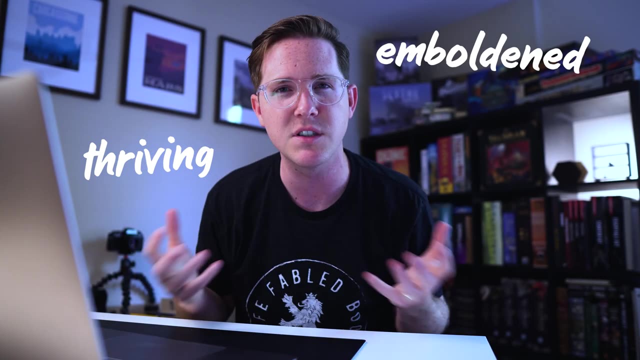 and that feeling is not about being stranded on a deserted island, forced to survive the elements. My game is not about survival. Instead, it's about thriving through the wilderness, feeling emboldened to explore and charting your own path towards completing goals that you've set out for yourself. 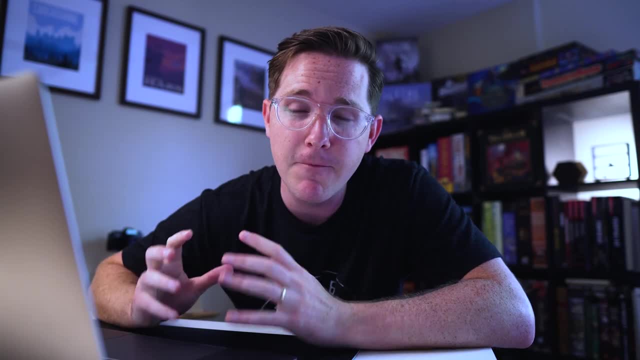 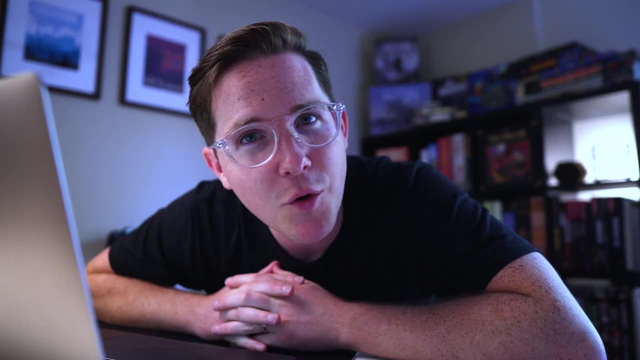 It is about challenge by choice. My game may seem visually similar because it uses hex, tiles, dice and cards, but I can promise you my game will feel very different. Those of you in the comments who've helped point out these games as good references, thank you. Seriously, it is incredibly handy when I ask for leads. 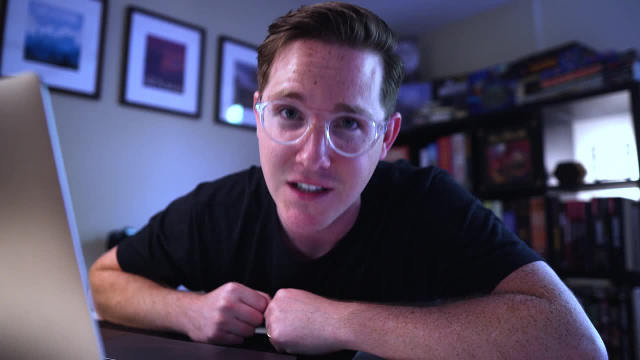 and suggestions that could help in my game design and you guys deliver. You're awesome, you're appreciated and you guys deserve it, Thank you. You probably know more games than me, so keep it up, but if you think that I'm 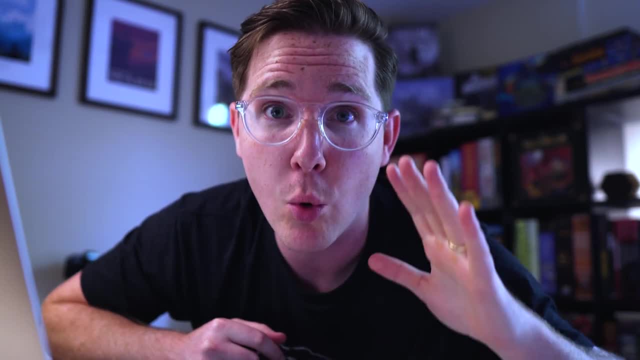 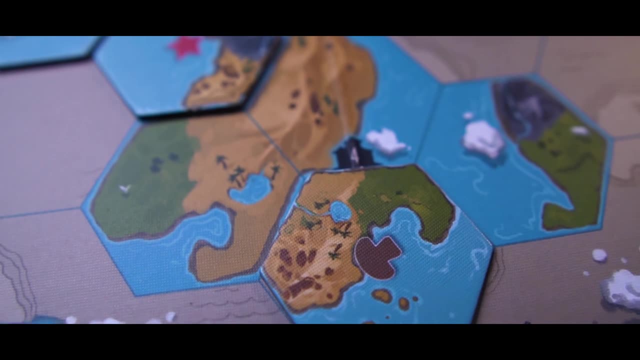 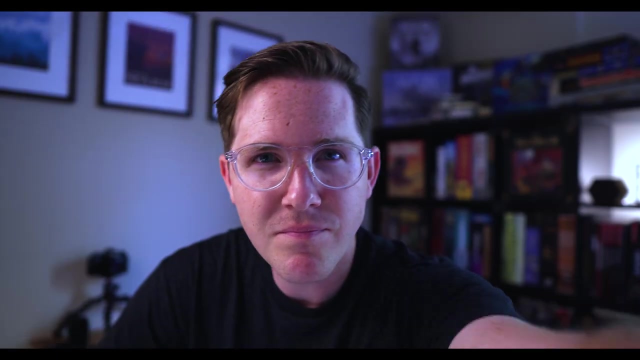 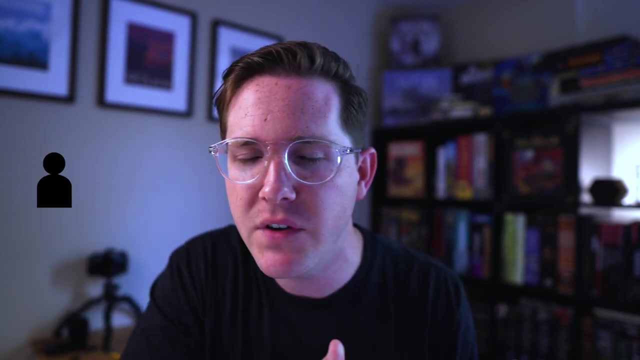 designing a game that's already out there right now. you better let me know right now. Okay, let's get into it. I'm claiming that my game will create narrative or perceivable story arcs for players to enjoy individually or collectively through the gameplay. 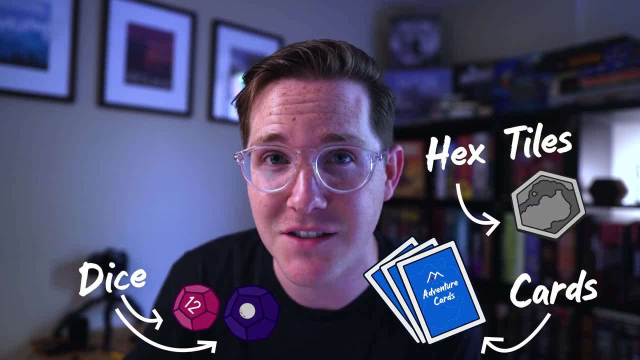 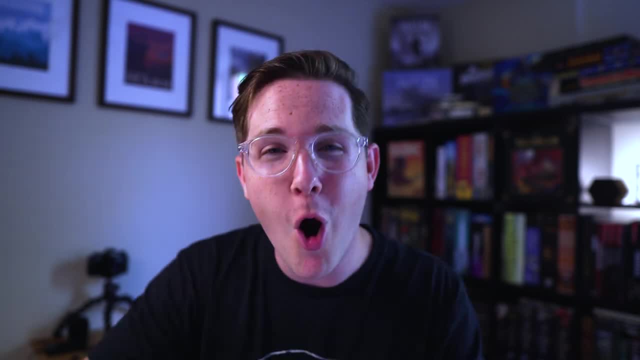 I believe that my game would create narrative by the way tiles, cards and dice are played. My players should see that there are layered events happening in the game that tie together through separate mechanisms and components, all reinforcing the theme of exploration and adventure. If everything works right, then 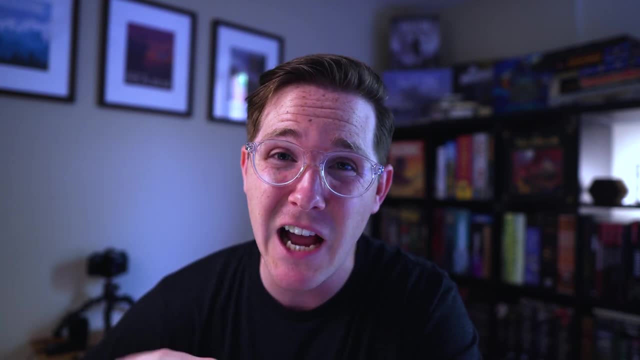 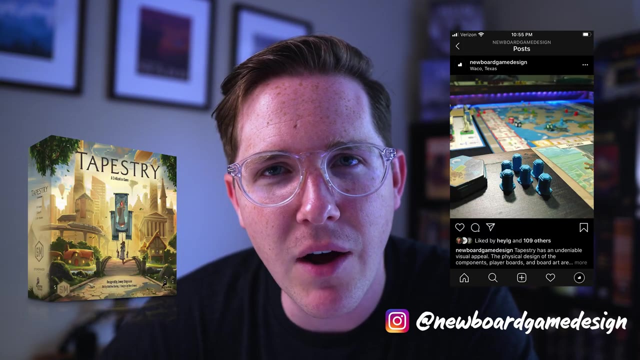 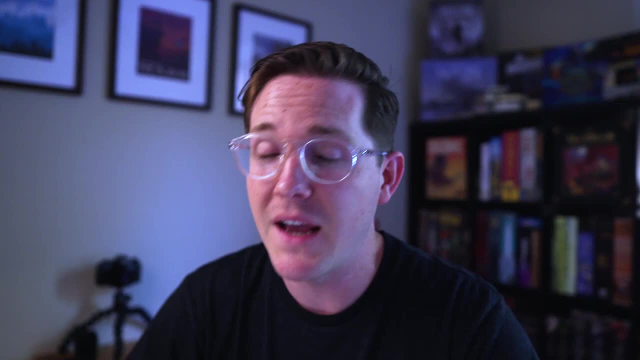 Tapestry makes me feel less like I'm building a civilization and more like I'm building a game. Tapestry makes me feel less like I'm building a civilization and more like I'm building a game. to them on each point. example number two: the cards and items. like many other games, i would 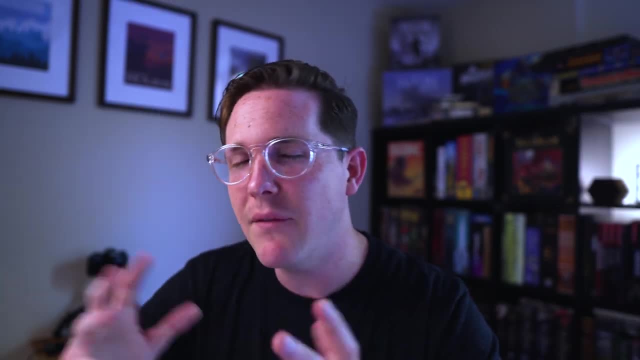 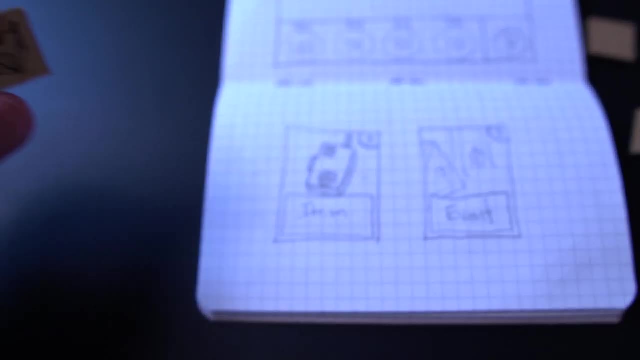 love for my players to find interesting things that would help them in the game. i have an idea that players will come across items on the cards that they're drawing from the adventure deck, but those cards, which give a description of the item, correlate to a physical token that you will place. 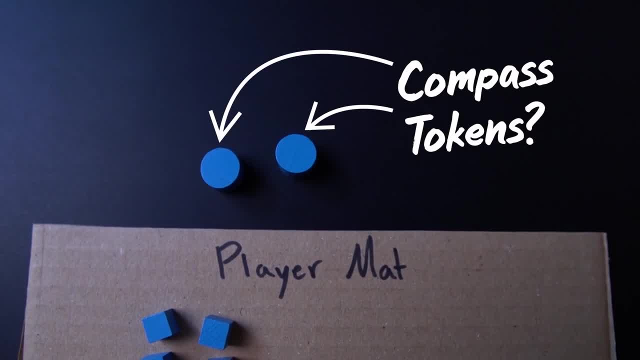 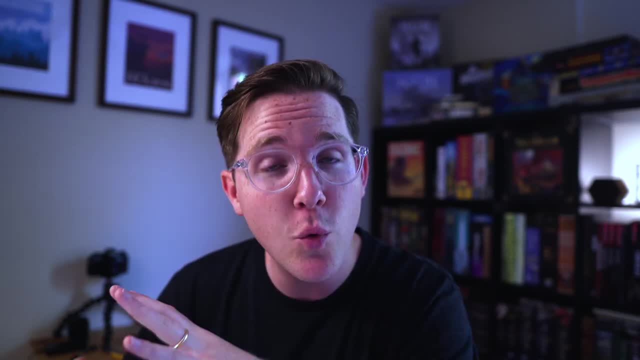 next to your player map so players can easily see the tokens and abilities all other players have in front of them. let's say, you draw an item card and that item is a functional walkie-talkie radio. since you found a walkie-talkie, you place a token next to your player mat so you don't forget and 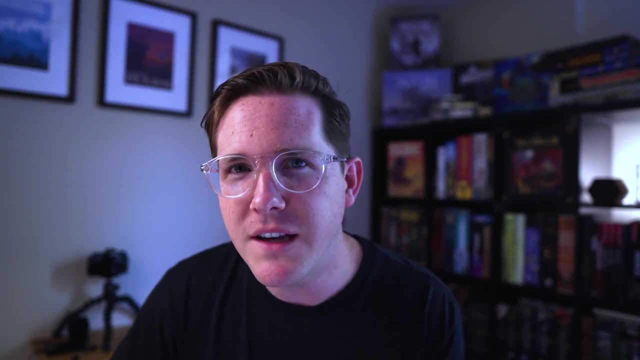 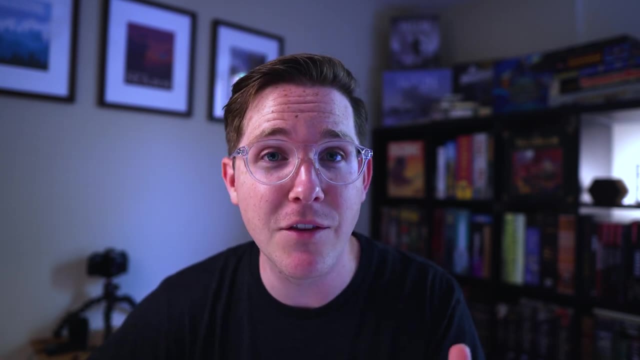 you rely on the card to tell you what the item allows you to do. what if walkie-talkies allow you to communicate to other hikers in the region that also have walkie-talkies? and, just like delilah in the video game firewatch, you are able to get advice on how to safely navigate difficult terrain. 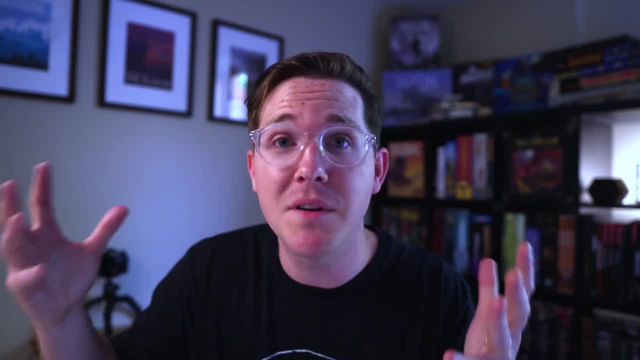 from any other hikers you can communicate to. you may have less compass tokens that limit your ability to ascend the mountain, but now you've found a radio that can take advantage of the compass tokens that other hikers can't access and you can use that to communicate to other hikers. 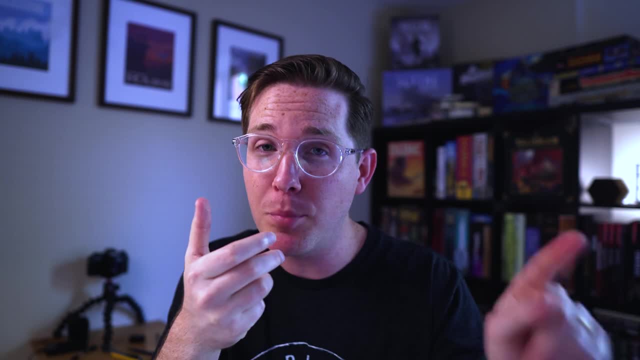 such as the radio, radio that can take advantage of the compass tokens that other hikers can't access players have in front of them, pretending that you're radioing in the other player's hiker as a virtual trail guide allowing you to benefit from the higher. 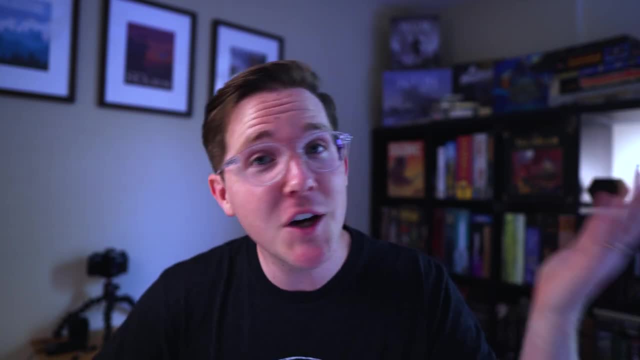 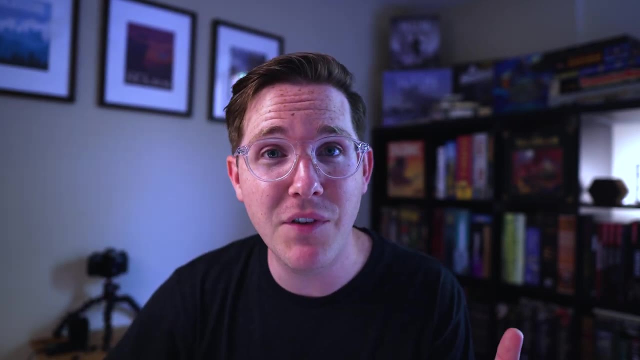 amount of compass tokens that that player has. Some players may feel frustrated that other players are taking advantage of their hard-earned knowledge, but the walkie-talkie is worth both ways. That player could eventually take advantage of your compass tokens later in the game At any point players could. 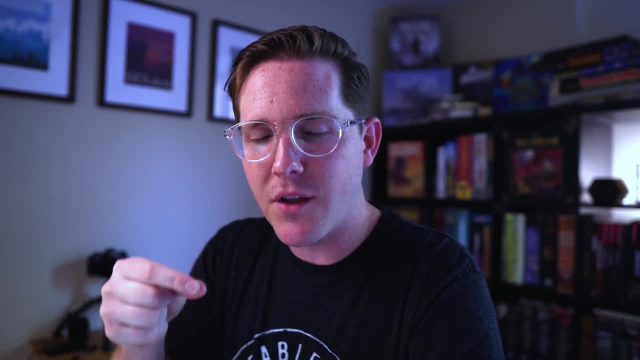 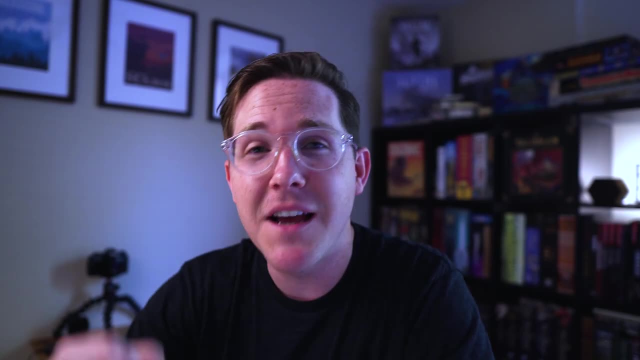 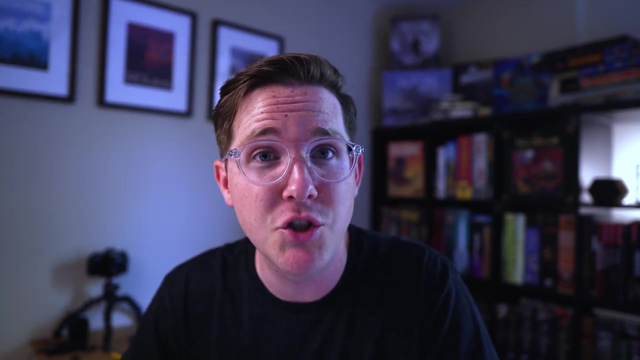 choose to discard their walkie-talkies, leaving them on the current hex space that they're on and eliminating the chance for other players to radio in and get their secrets. Example number three: risk and lost items. The mountains are a dangerous place, Even at the base of a mountain canopied by trees and 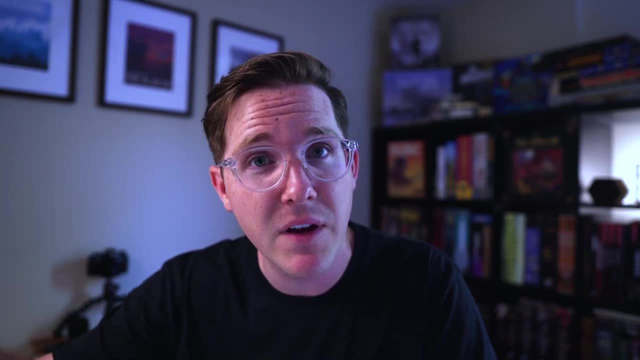 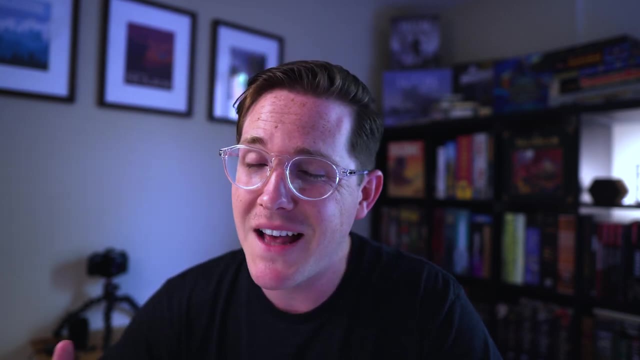 vegetation can be precarious sometimes, depending on how steep the face is and how unstable the ground can be for secure footing. I want players to have a healthy fear of ascending the mountain in my game because that matches the reality of my theme. Remember, I'm not designing a survival game, so no one's 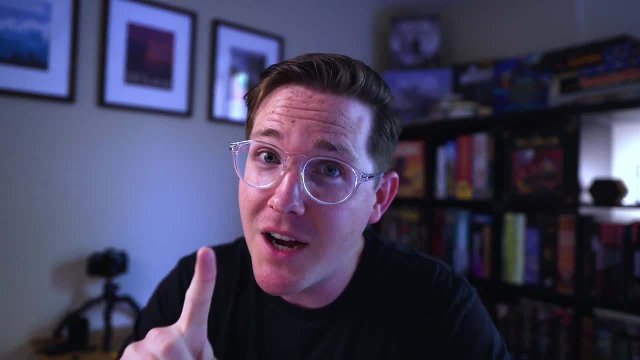 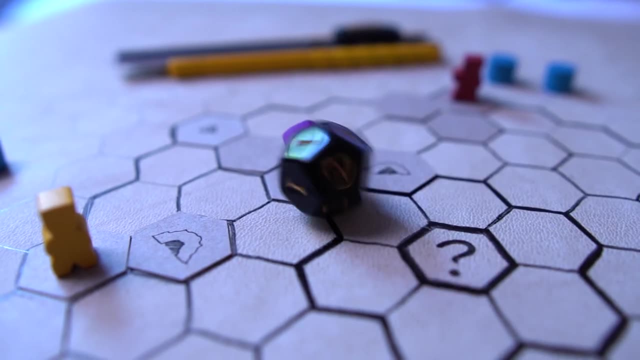 gonna be dying from falling off the ridge of a mountain in my game, But there will be consequences if a player falls off the ridge of a mountain in my game. If a player decides to start their ascension committing to the risk of danger and they end up not making it, If they fail the attempt to ascend to the. 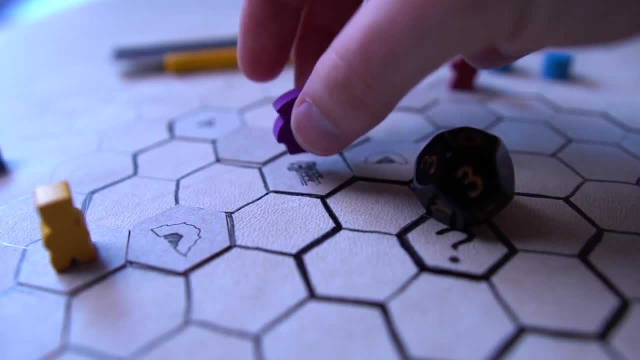 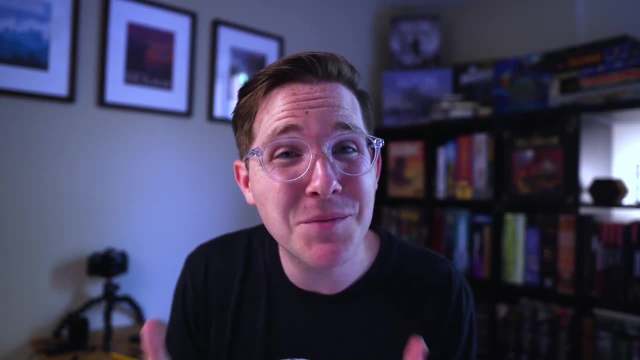 next available hex space. then they end their turn without progressing to another hex tile and they are forced to lose one or two items they've found along the way. Pretty low stakes for falling down a mountain, right? Well, what if you desperately needed those items for future turns, and now they've been? 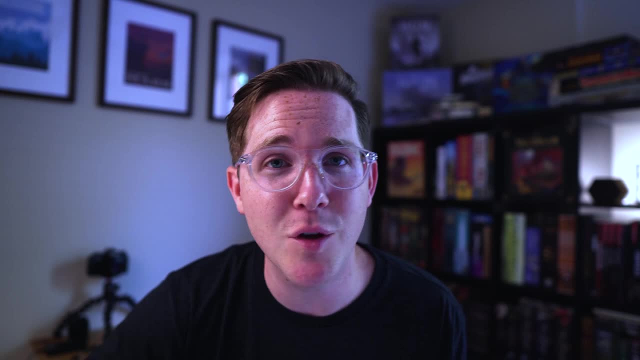 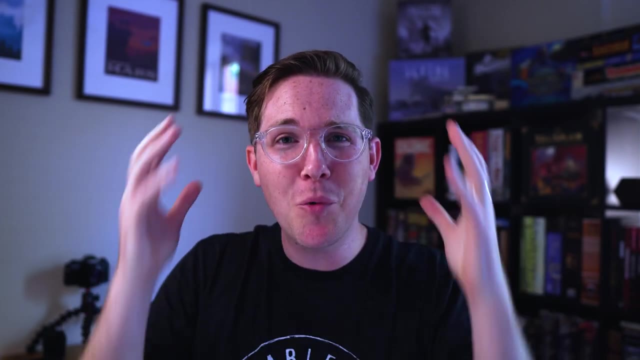 lost to the discard pile. There may only be minimal ways to regain those tokens: by exploring more and eventually coming across them again in the adventure deck. Oh, if only you would have waited before you had one more compass token, and then you would have made it. 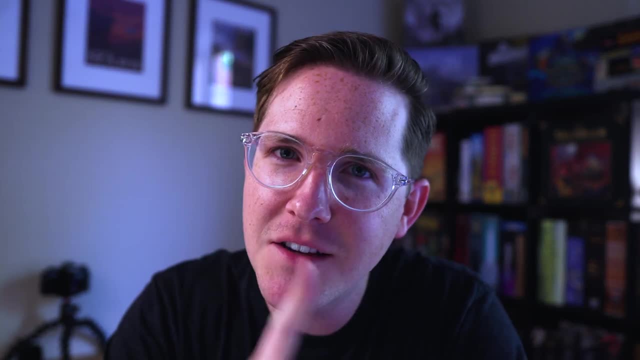 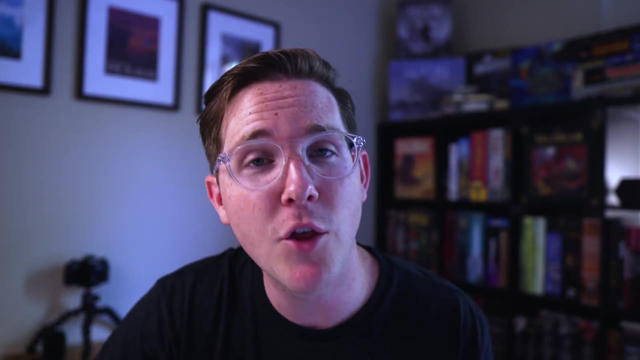 and not lost your dang walkie-talkie. You see how that could be a narrative moment. Yes, it might suck that you have less chance to win the game now, but it was your choice all along and you and the other players will remember that.